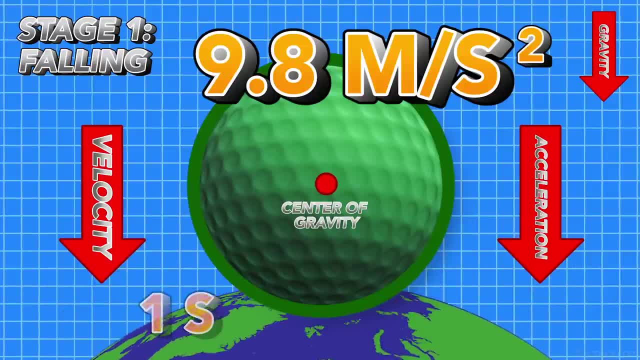 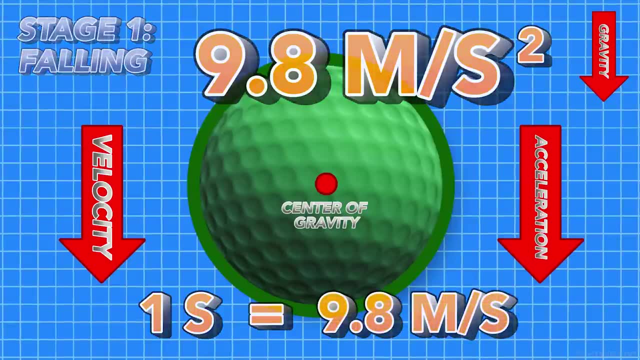 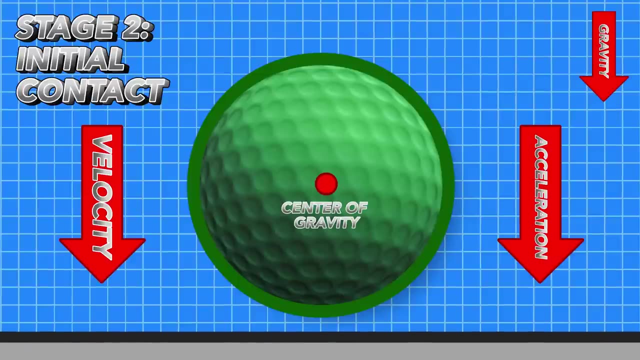 due to gravity is 9.8 m per second squared. This means in essence that for every second of falling, the ball's velocity will accelerate by 9.8 m per second. The next stage is initial contact. The initial contact phase is just that when the ball 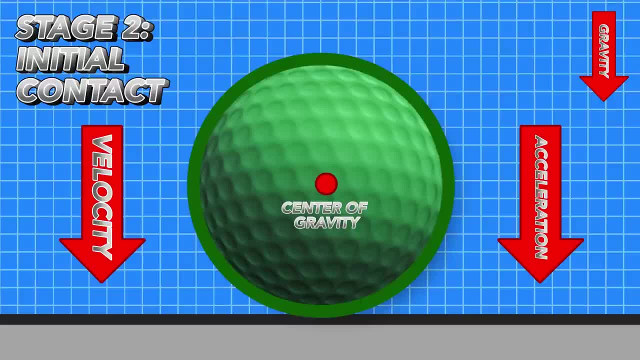 just barely makes contact with the ball. This is called initial contact. That means that the ball is just barely making contact with the ball. The next stage is initial contact with the ground's surface. It will continue to fall under the influence of gravitational acceleration, but now a normal force from the ground's surface. 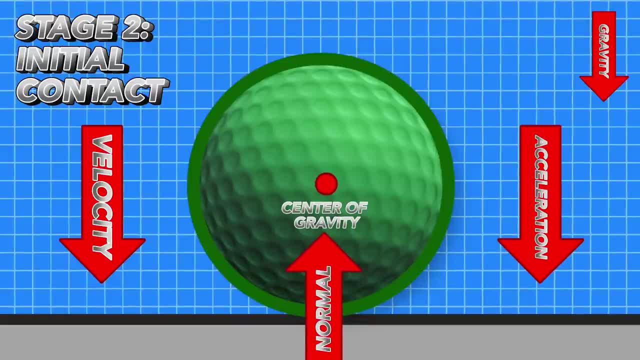 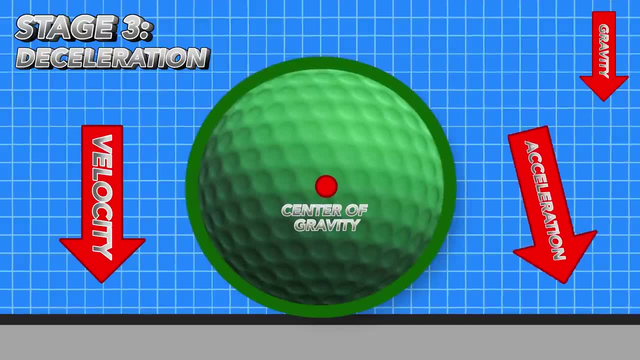 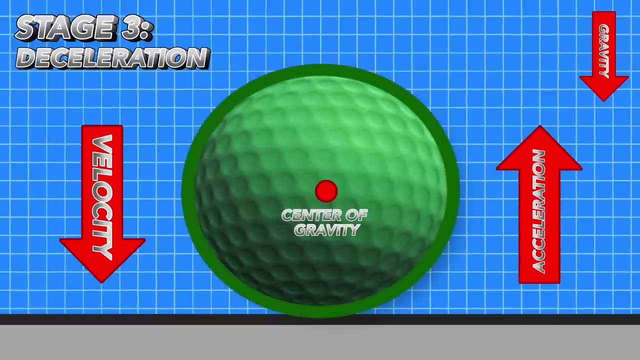 opposing the force due to gravity will act on the ball. Next we have deceleration or negative acceleration. After initial impact, the ball rapidly decelerates, or rather accelerates in the negative direction. The velocity of the ball still points downward as it deforms, but acceleration on the ball is. 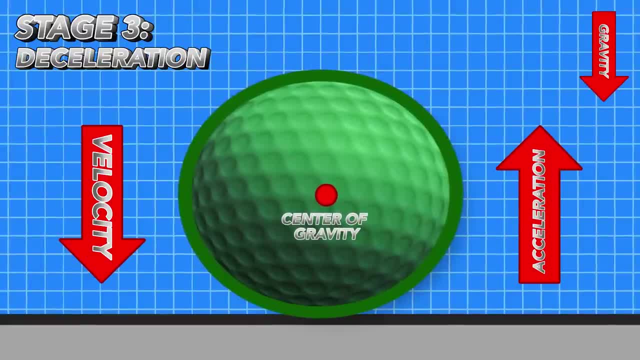 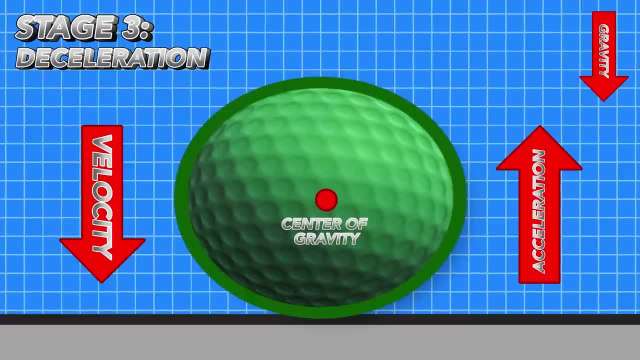 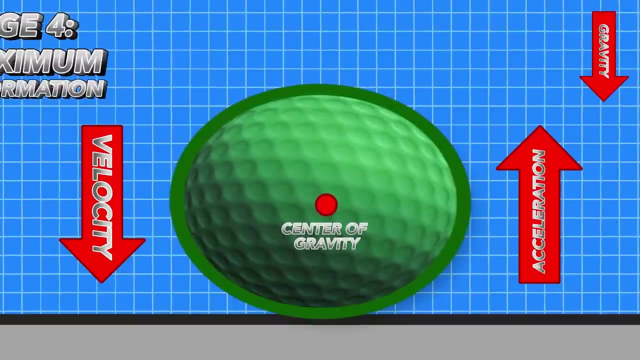 beginning to point back upward as the forces from the reaction overcome gravity. This all means that the ball is pushing on the ground with a force that is greater than its own weight, so acceleration must point upward. Following the deceleration stage, the ball has now reached the maximum deformation stage At 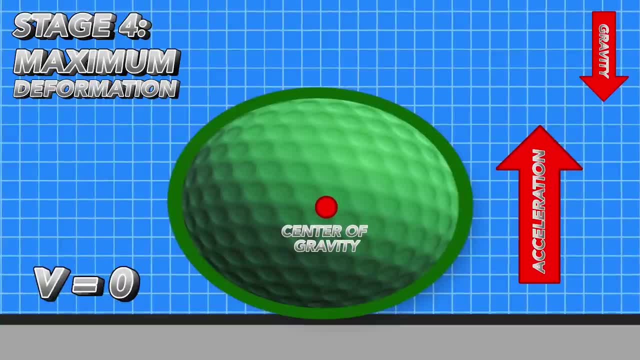 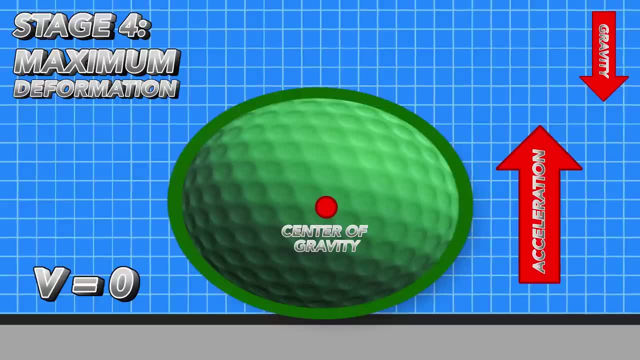 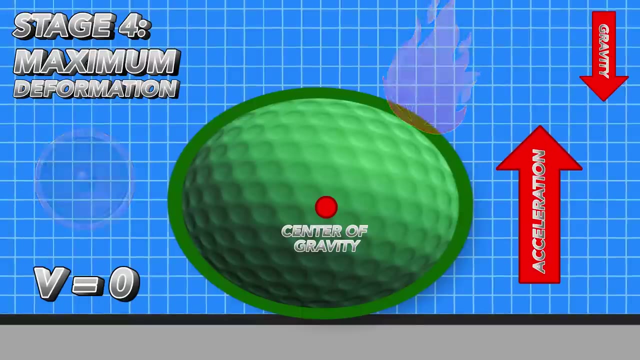 this point, the velocity is zero and the acceleration vector points upward. This is the lowest point of the ball, as well as its maximum deformed point. If we assume the ball to be totally elastic and ignore other energy losses like sound and heat, the ball would bounce back up to its original drop. 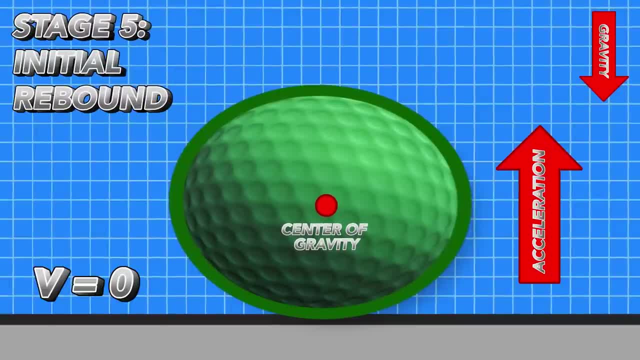 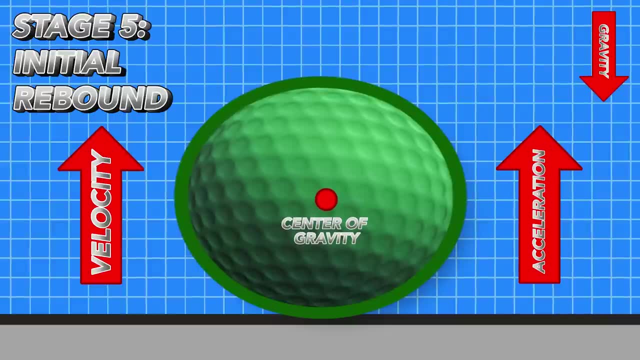 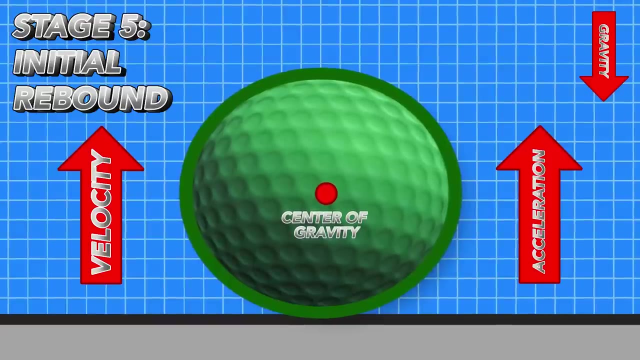 height after this point. Now we've entered the initial rebound phase. This stage begins the ball's journey back to where it began. Its velocity and acceleration vectors are pointing in the same direction, meaning upward movement. The ball is less deformed than the maximum deformation stage and, due to its 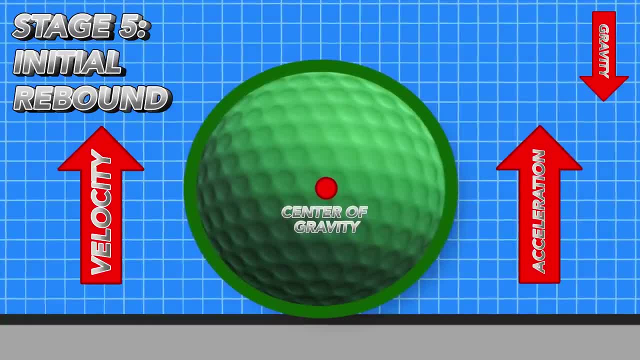 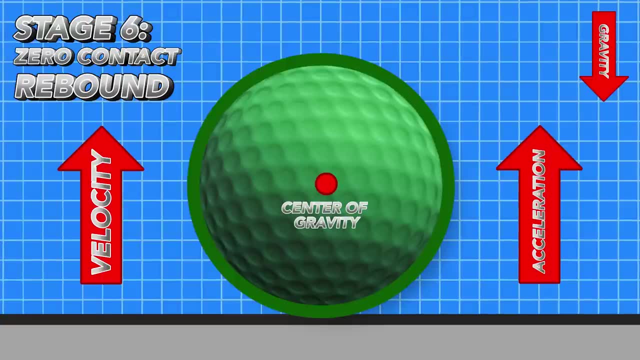 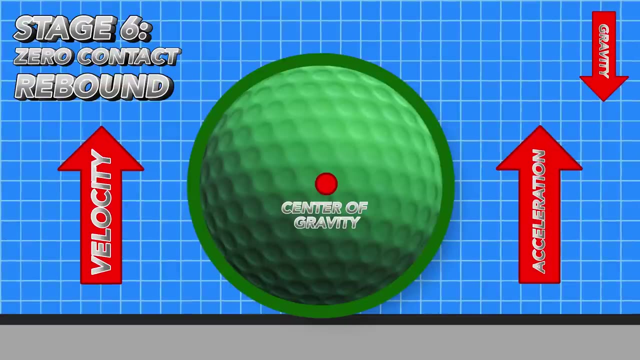 force, pushing against the surface with a force greater than its own weight. this is what will cause the ball to bounce upward. Now we've reached the sixth stage, the zero contact rebound. At zero contact rebound, the ball is no longer deformed and is barely touching the surface, essentially only at one point: Velocity is. 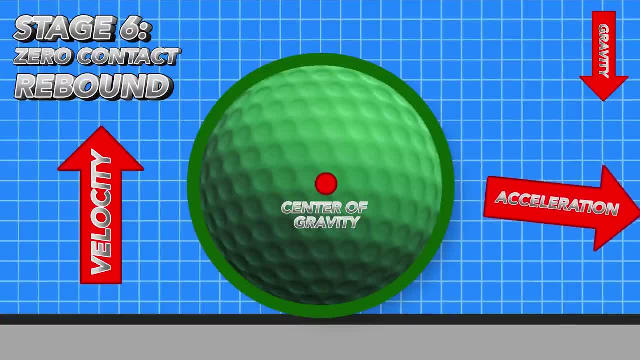 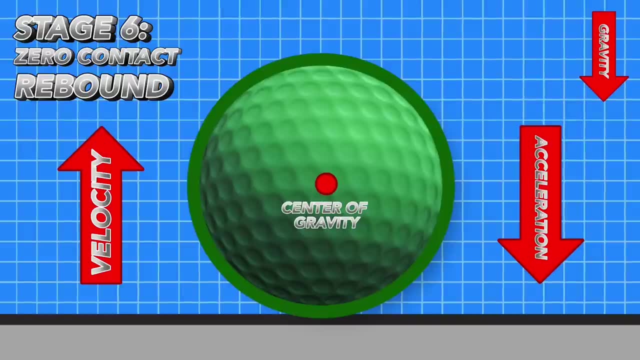 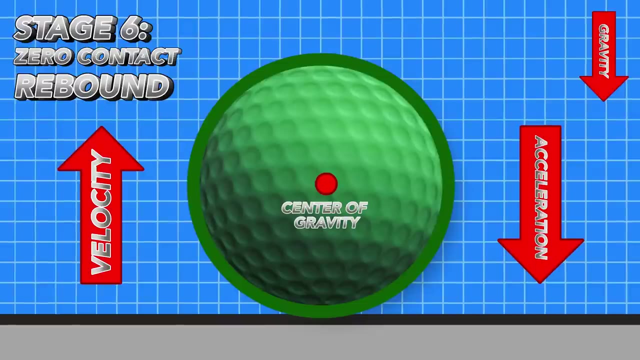 moving the ball upward, but at this point acceleration switches to oppose the velocity vector. This is because there's no longer any force from the elasticity of the ball pushing on the surface giving it an upward acceleration. Acceleration due to gravity, which pulls downward, will now be the only force acting on the ball in a 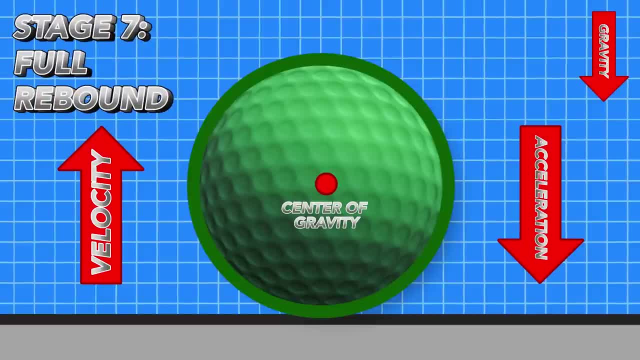 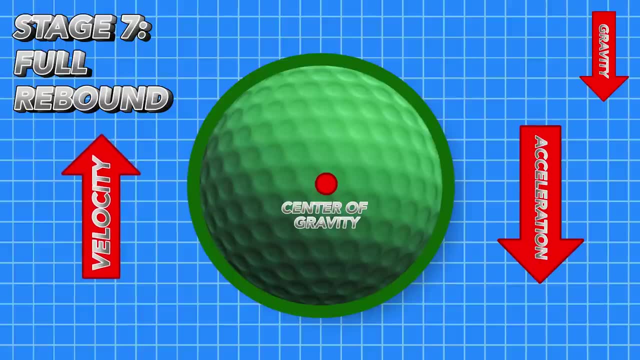 perfect system. And the final stage, full rebound. At full rebound, the ball has left the surface and its velocity vector still points upwards, though shrinking steadily due to the acceleration or deceleration due to gravity Following this step. the ball will reach a peak at a new step, one where its velocity vector 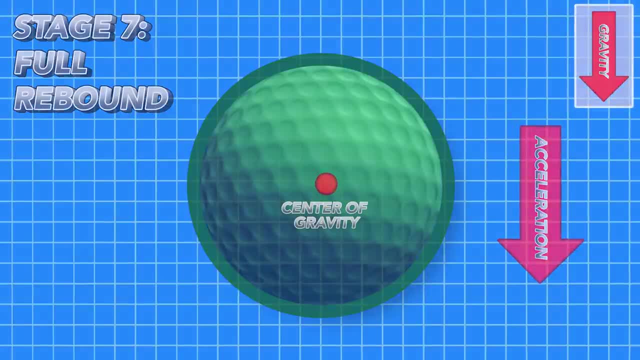 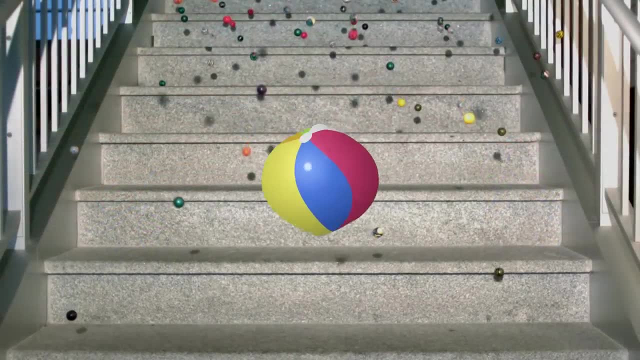 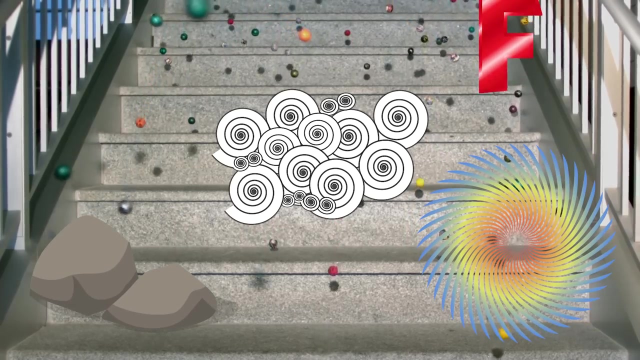 is zero and the only force acting on it is gravity. Now we can start to look into adding variables in special cases in bouncing ball physics. This previous case of the bouncing ball was simplified to remove any other forces like air resistance, imperfect elasticity, spin, friction and force from an initial 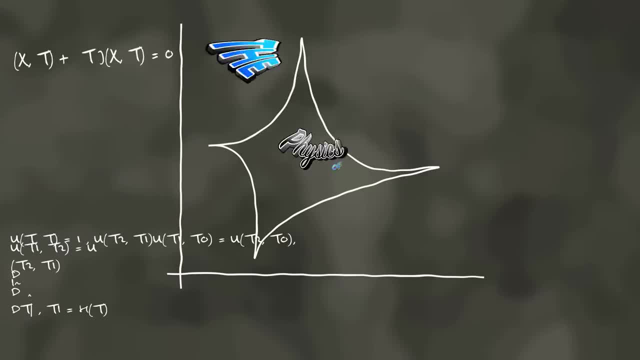 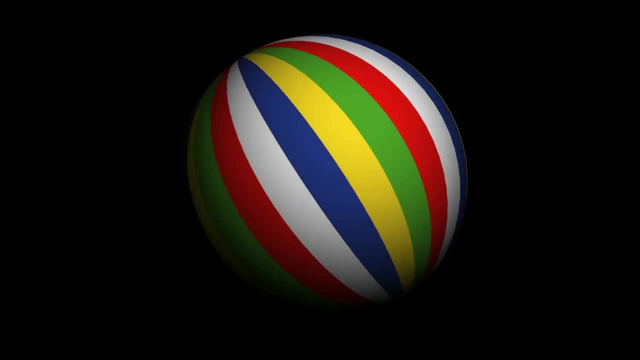 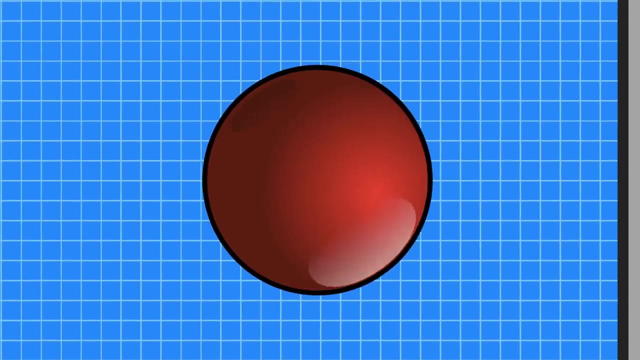 throw, among others. All this means that bouncing ball physics gets more complicated from here. When balls have any spin, as they usually do when thrown, and and when the surface they hit isn't frictionless, the ball's spin reverses from before to after impact. 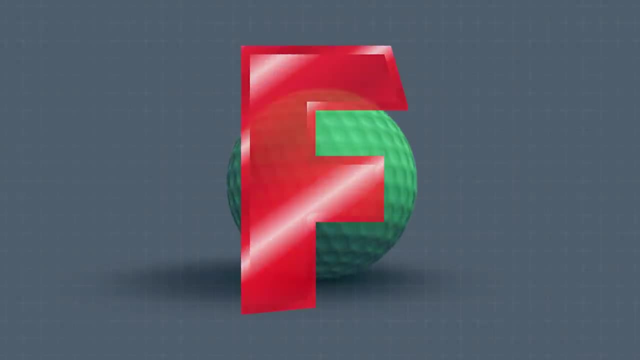 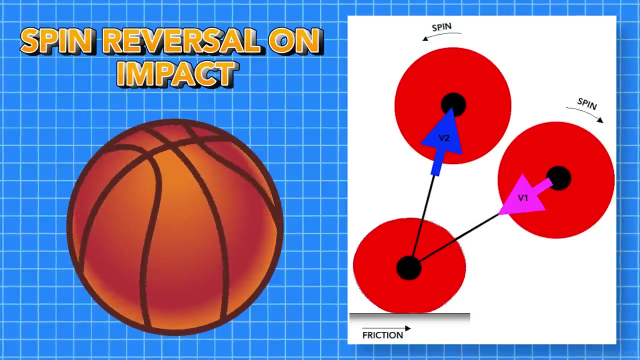 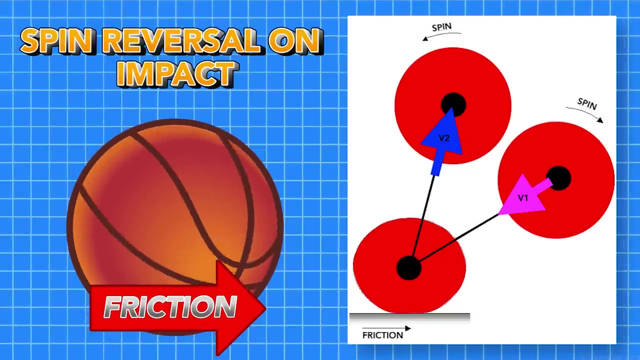 This is actually due to the force of friction. Assuming two dimensions for theory's sake, you can observe the reaction here: As the ball impacts with a spin in one direction, the friction force F counteracts the ball's spin, or rather, the friction force is always opposite. 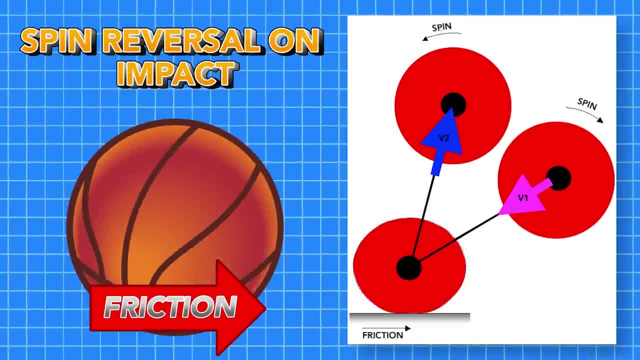 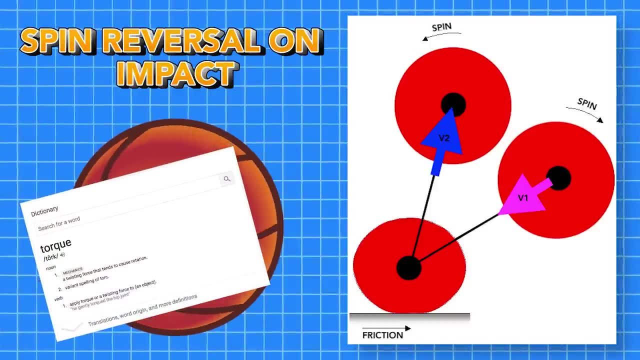 the direction of the slip velocity between the spinning ball and the surface. Since the friction force is opposite of the ball's spin, it torques the ball in the other direction. It also causes the path of the ball's bounce to skew in the direction of the friction force. 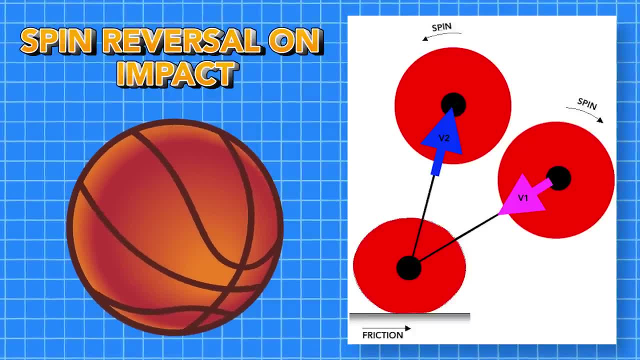 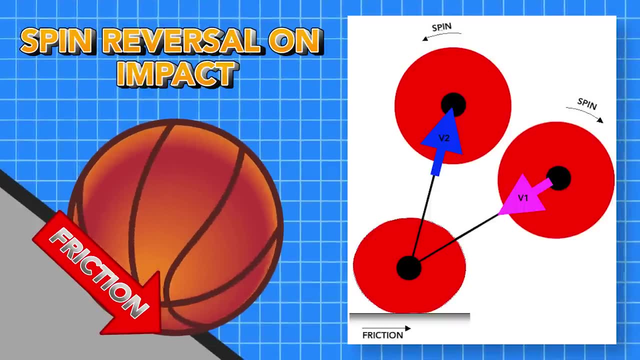 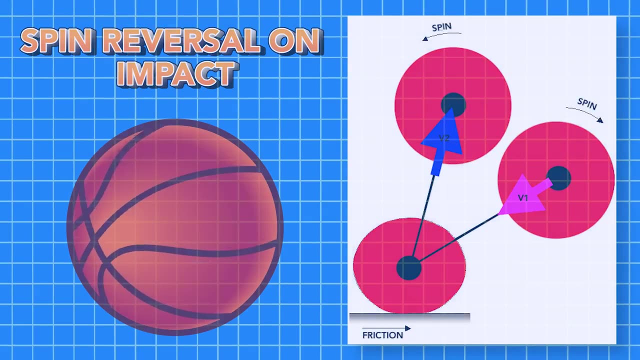 In simplified terms, when a ball spins in one direction, when it hits a wall, the friction between the ball and the wall overcomes the spin so much that it reverses its spin direction. This spin reversal doesn't happen if the ball and the wall's coefficient of friction isn't high enough. 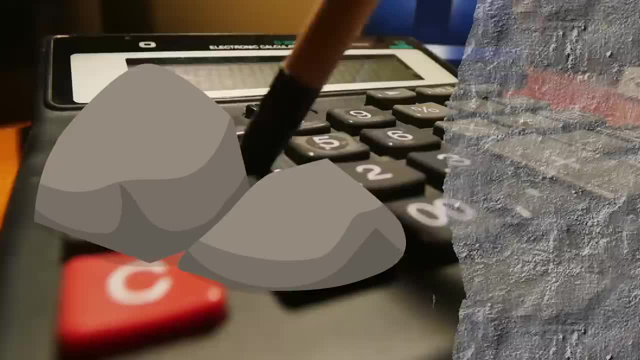 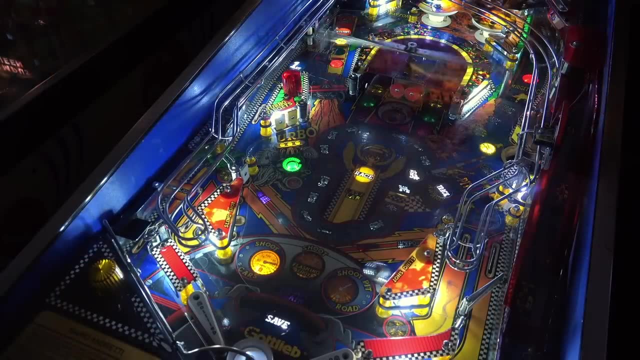 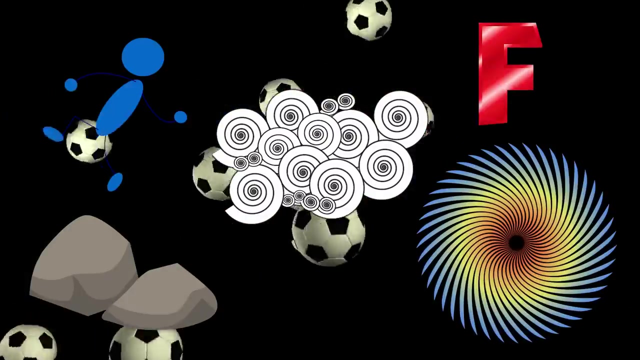 The coefficient of friction varies by material and surface and is essentially a number that indicates how grippy a surface or material is. In real, non-ideal scenarios, bouncing balls lose energy and eventually come to a stop. This is all due to the forces we ignored. 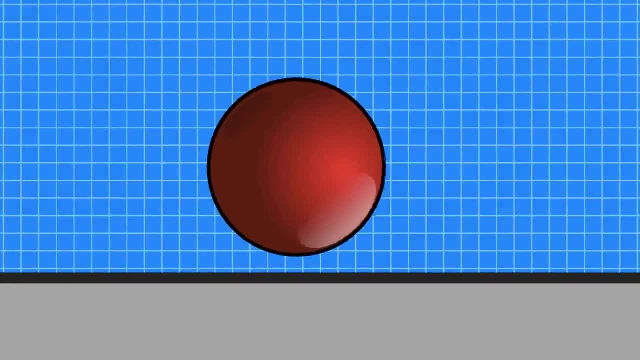 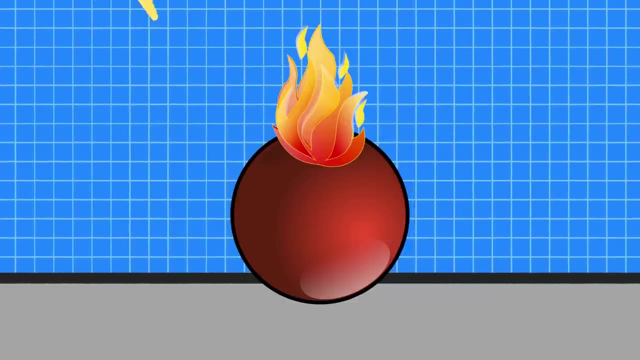 in the first example, When a ball hits a wall or surface, it makes a noise, which is a loss of energy. from the ball's bounce It will also generate some amount of heat- another loss of energy: Friction from the wall will also cause energy loss.